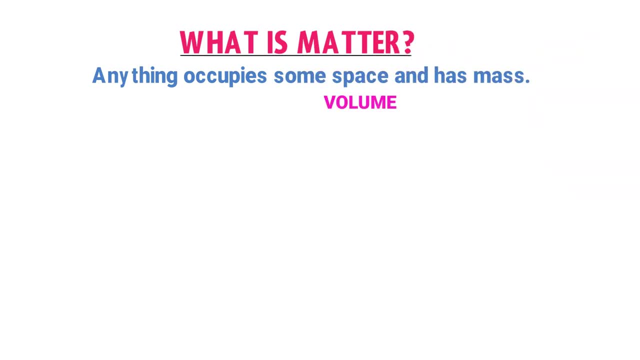 means volume and has some mass, is known as a matter. For example, a cup, a desk, a car, etc. This cup has some mass and volume. Similarly, this desk and this car also have well-known masses and volumes. Thus, anything around us having some mass and volume is called matter. 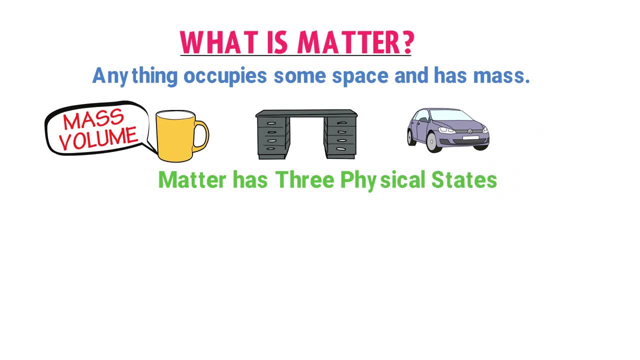 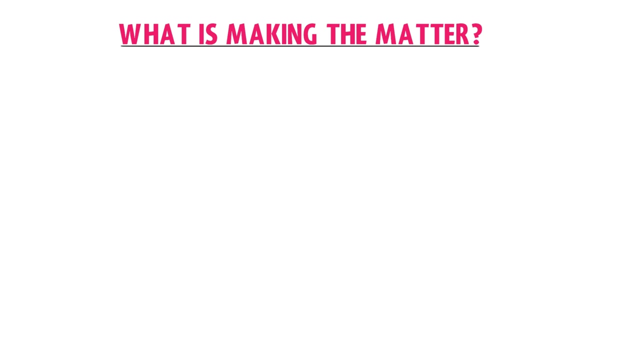 We have also learned that matter exists and three physical states: solid, liquid and gas. For example, a cup is a solid, water is liquid and air within the balloon is gas. Here, the important question is: what is making the matter? To learn this question, you should ask that: what is making the wall? 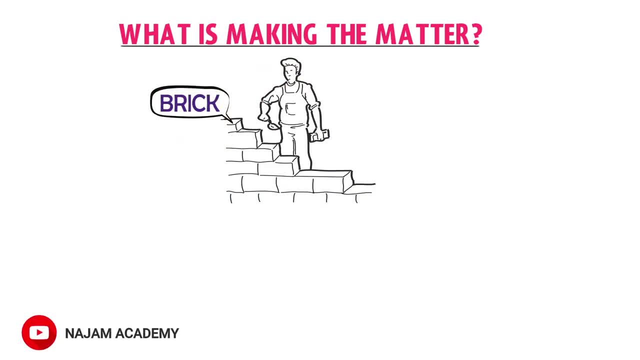 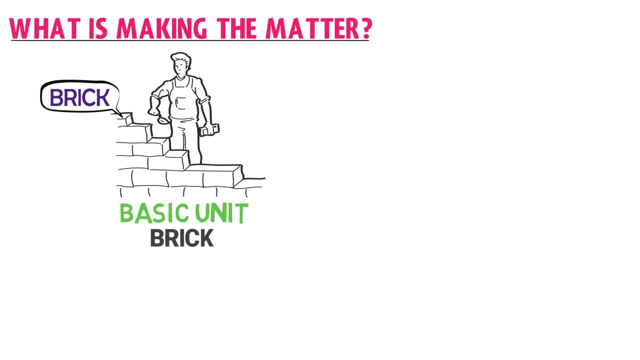 Well, the answer is: it is the brick that is making the wall. Or you can say that the basic unit of this wall or any house is a brick. Similarly, matter is made up of atoms. For example, this cup is a matter. It is made up of millions of atoms. Hence we say that the basic 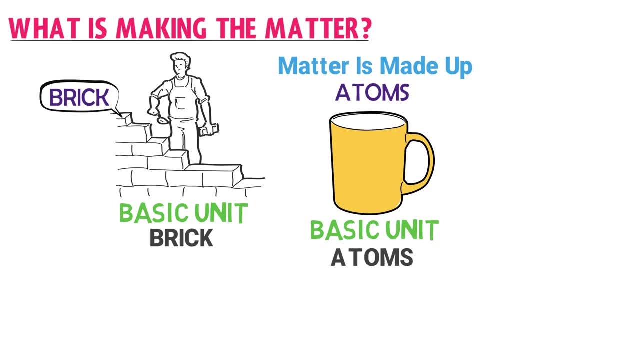 unit of matter is an atom Or it is atom that is making our consciousness? We know that there is cement that is holding together all the bricks of this wall. Here is the important question, As I told you that this cup or this matter is made up of millions of atoms. 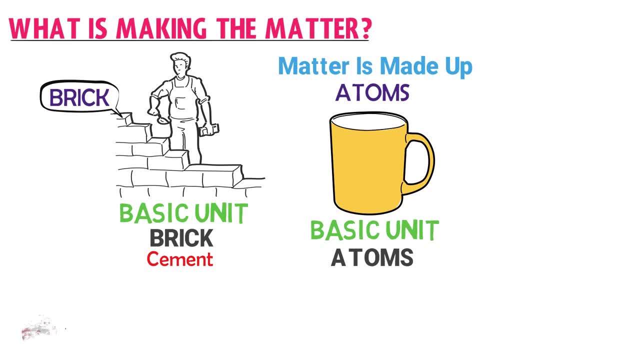 Now, what are holding the million atoms of this cup? Well, just like cement that is holding together all the bricks, there is chemical bond That is holding together all the atoms of the cup, or matter. One can say that there exists chemical bond between two atoms. Let's consider two atoms of this cup. We know that these two 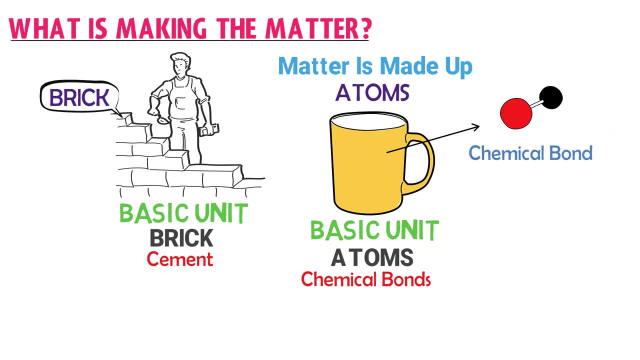 atoms of the cup are joined together by a chemical bond. Due to this chemical bond, there is living or present chemical energy. Remember that when there is chemical bond, there is energy. Now just imagine there are millions of atoms in this cup. Thus there will be million chemical. 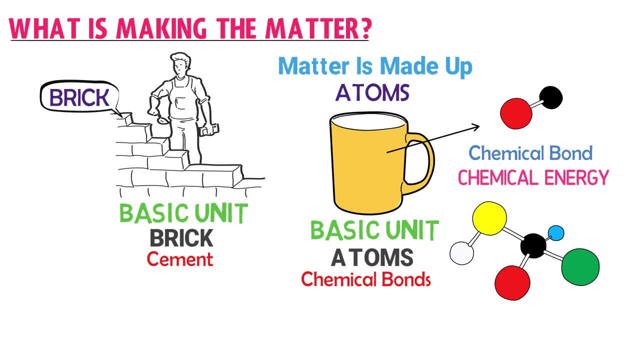 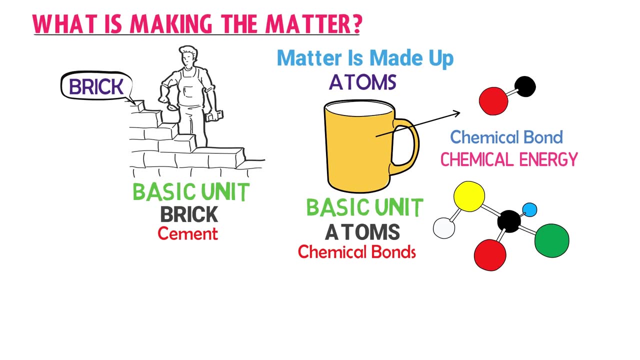 bonds, And you can just think about the energy present between these chemical bonds. Hence, we can say that this cup is a matter. This matter possesses large amount of energy due to chemical bonds. Therefore, we say that when there is matter, there is energy. 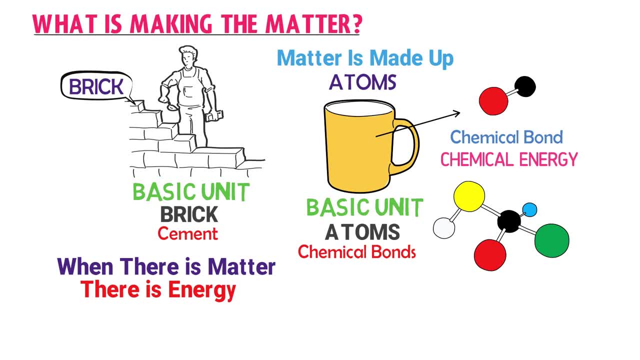 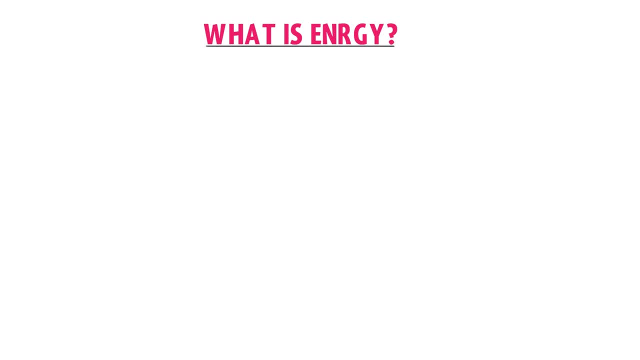 Let me repeat this important statement: When there is matter, there is energy. Now, what is energy? Energy is defined as the ability to do some sort of work, is known as a energy. For example, you need energy to walk, you need energy to talk, you need energy to grow. a car needs petrol which contains chemical energy to run. 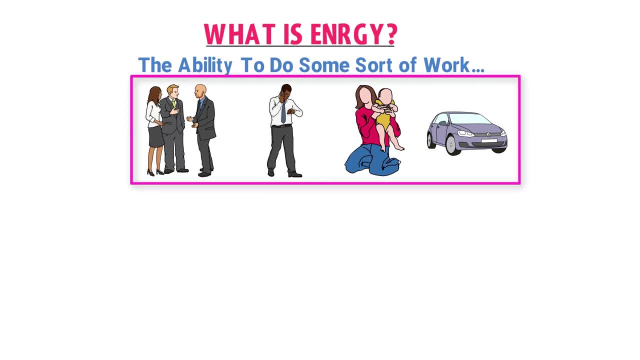 Thus, we all need energy for doing different jobs or work. Without energy, no work done is possible. Without energy, no work done is possible. Remember that energy exists in different forms. For example, if an object is raised above the earth's surface at certain height, 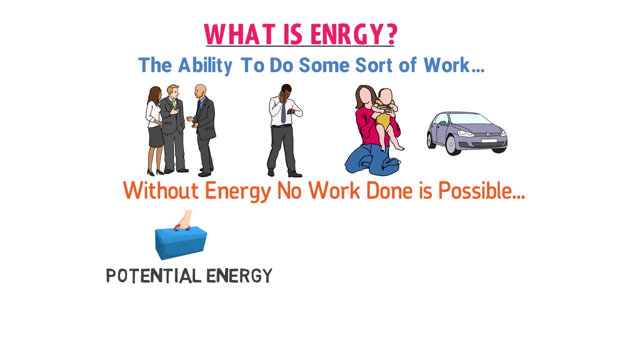 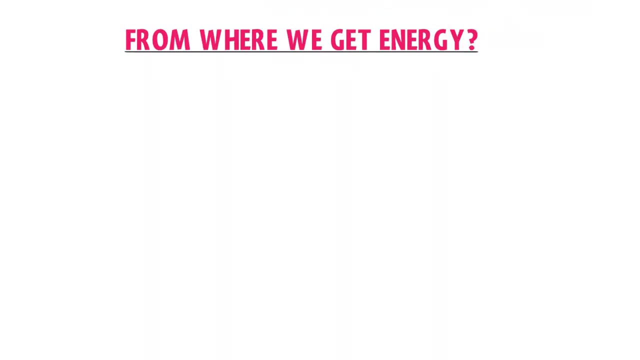 this object possesses gravitational potential energy. Similarly, a fast-moving object possesses kinetic energy. Due to its lack of energy, it does not produce a gravitational energy motion. the another question you must learn is that from where we human beings get energy? the answer is simple: we get energy by eating different types of food. 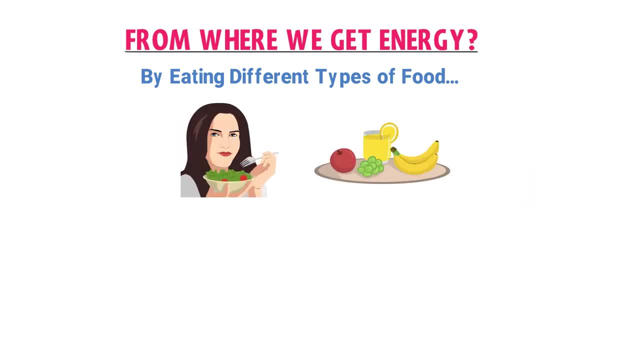 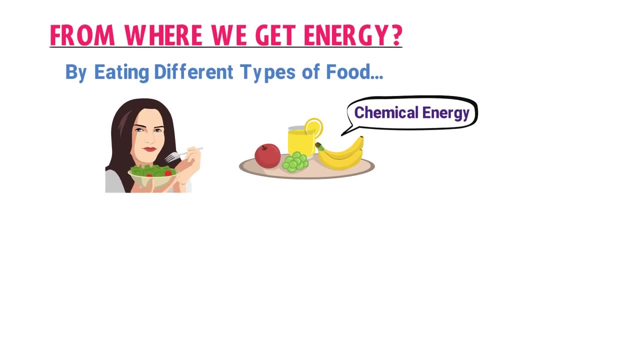 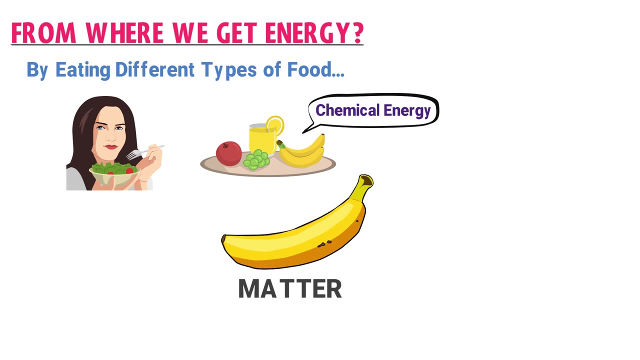 for example, we get energy by eating vegetables and fruits. the fruits and vegetables we eat contain chemical energy. let's consider you eat a banana. we know that banana is matter because it is made up of millions of atoms like carbon, hydrogen, etc. atoms of the banana are joined together by chemical bonds. we 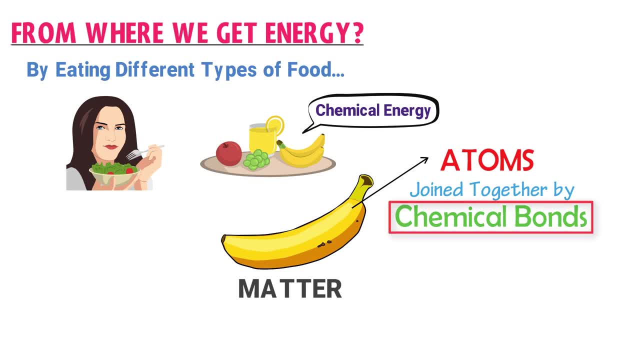 learned in the previous slide that when there is chemical bond between any two are more than two atoms, there exist energy. capsules are chemical energy. this banana possesses chemical energy one. Once you digest the banana, you get chemical energy and then you can convert this chemical energy into other forms of energy, like sound energy, kinetic energy, potential energy, etc.